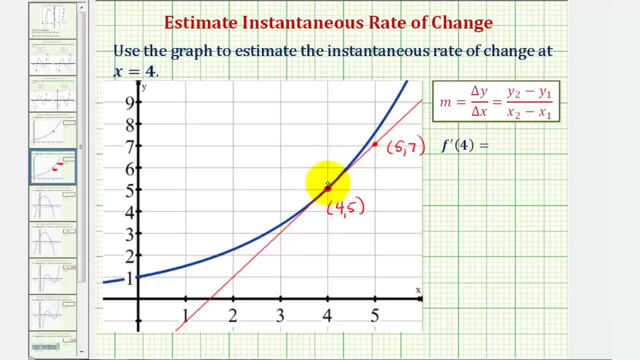 to the point on the right, we would have to go up two units, which means the change of y is positive two, And then we'd have to go right one unit, so the change of x is positive one And therefore the instantaneous rate of change. 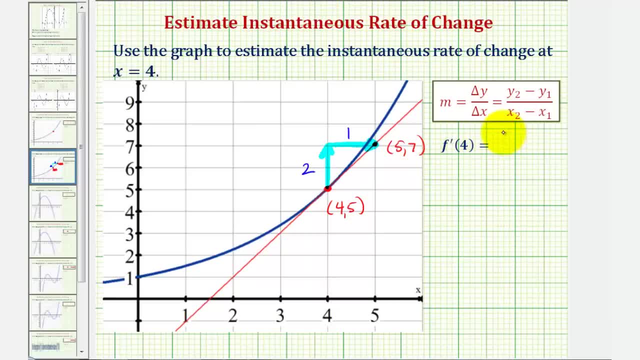 at x equals four or f, prime of four is equal to two divided by one or just two. The other option is to use these two ordered pairs and find the slope using this formula. here again, where we have the change of y, 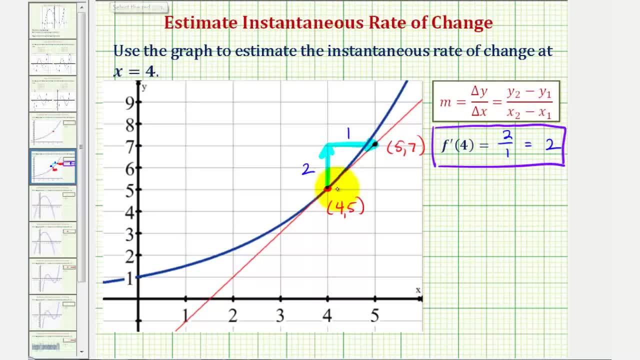 divided by the change of x. So let's also show that. Let's call these the ones meaning x sub one, y sub one. We'll call these the twos, meaning x sub two, comma, y sub two. So we'll get the same result. 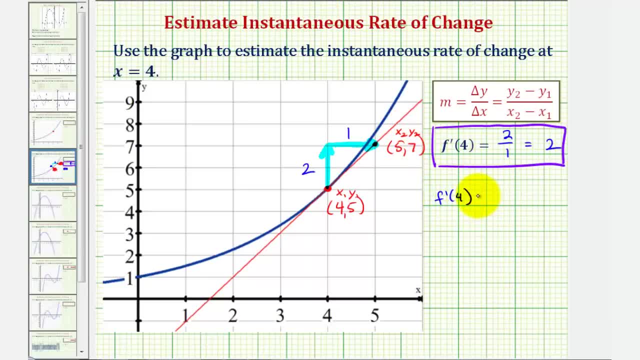 but f prime of four, or the instantaneous rate of change at x equals four, is equal to y sub two minus y sub one, that's seven minus five. divided by x sub two minus x sub one, that's five minus four, which gives us two over one. 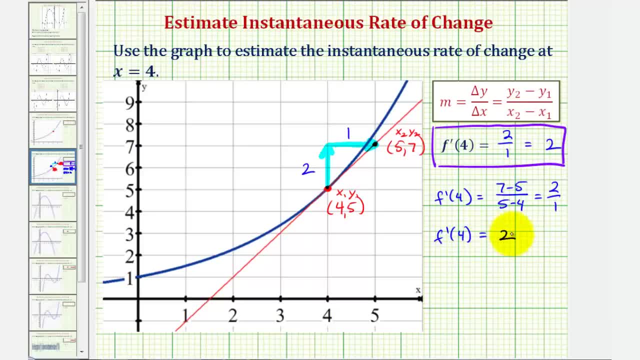 or, as we had before, positive two. To understand what this means, though, it's simple to have the instantaneous rate of change in fraction form, in this case two over one, So if f prime of four is equal to two over one. 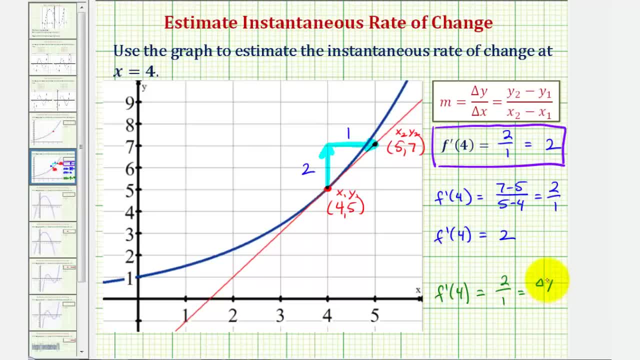 where the two represents the change of y, the change of function values- and the one represents the change of x. this tells us that when x equals four, the function value, or y value, is changing at a rate of two units per one unit change in x. 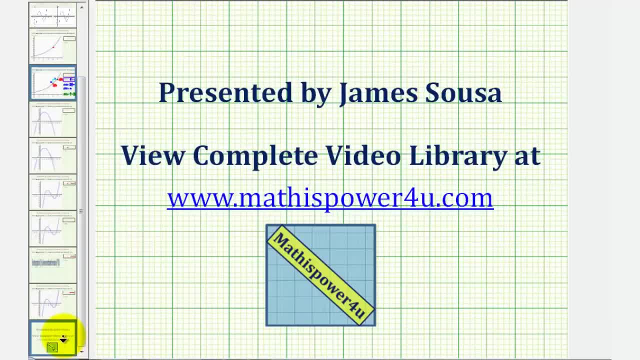 I hope you found this helpful. Thank you. 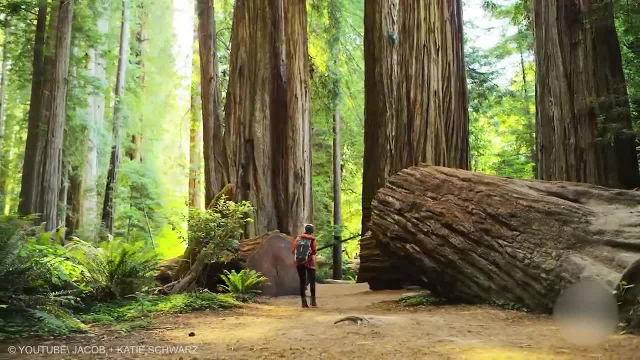 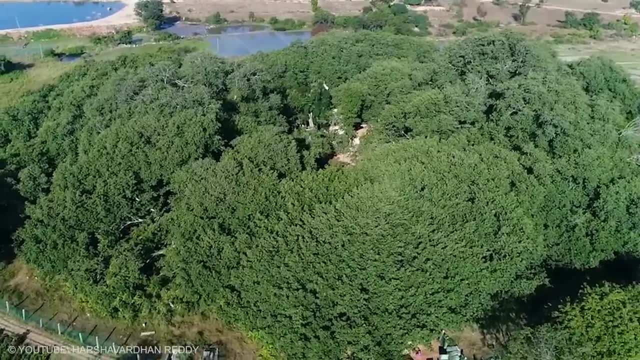 Trees are life-givers for many reasons, but few of them are recognized for their height. You'll probably be surprised at how big trees get, from the tallest types of trees in California to the largest canopies in India. Let's explore the oldest, tallest and biggest trees in the world.